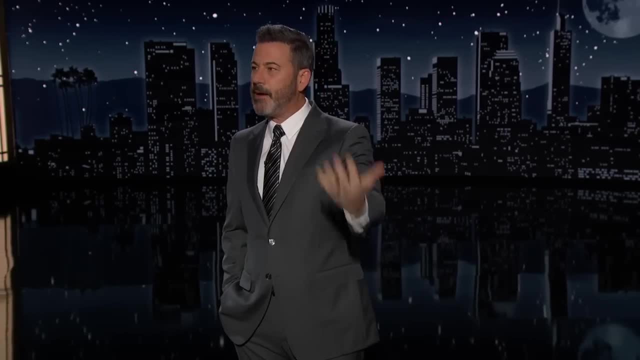 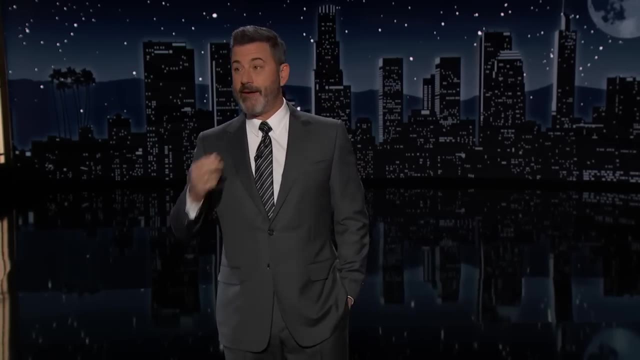 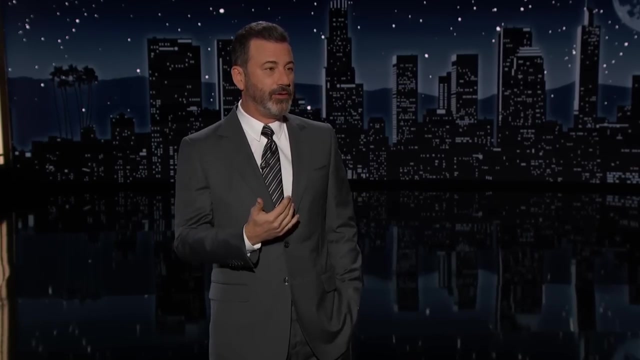 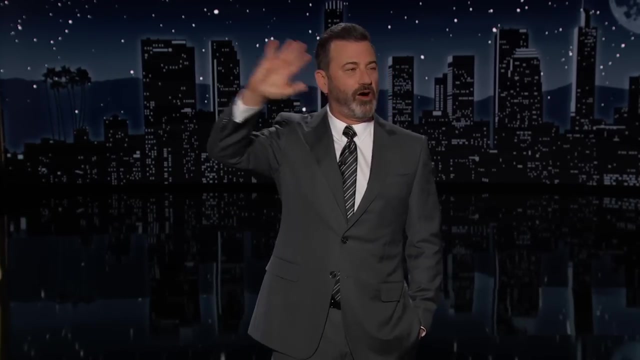 Welcome to the show. Thank you for watching. Thank you for coming on. Thank you for taking shelter here in our. well, that's very kind, I have to say. I want to apologize to our visitors from other towns We had. I hope you had a good week. We had some crazy, crazy weather here. I woke up on Sunday a huge piece of lattice had flown off my roof and onto my car, And that wasn't even the number one weirdest thing that happened. I had like 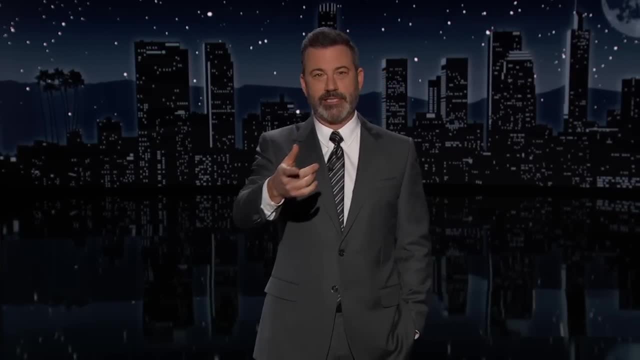 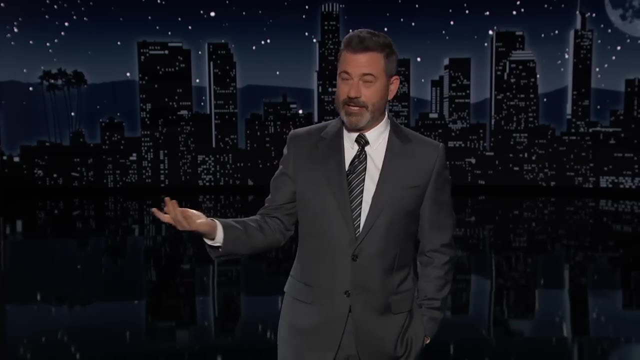 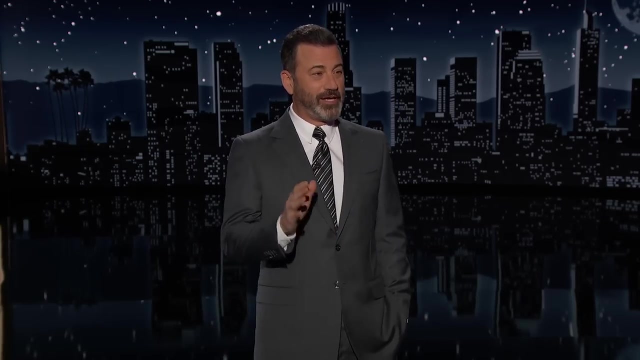 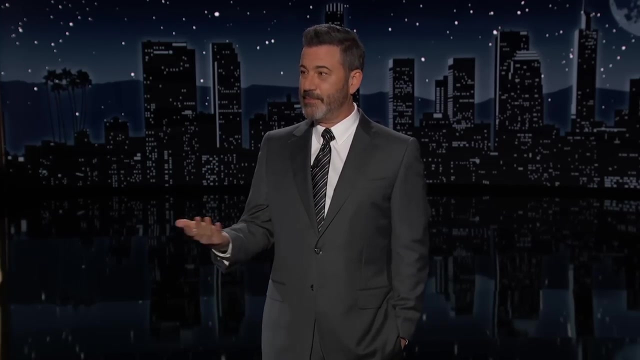 80 texts when I woke up sending me this article from Rolling Stone. It says: Trump White House pressured Disney to censor Jimmy Kimmel. Now Disney is the company that owns ABC, our network, and Jimmy Kimmel is me, So obviously I was interested in seeing what it was. But according to the story, in 2018, Donald Trump, who was at that time president of the United States, was so upset about my jokes that I made about him. he directed his staffers at the White House to call Disney. 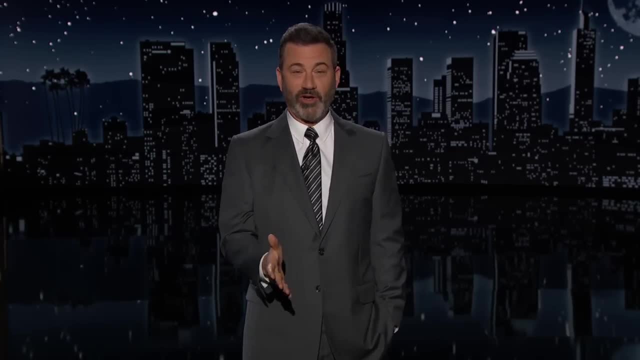 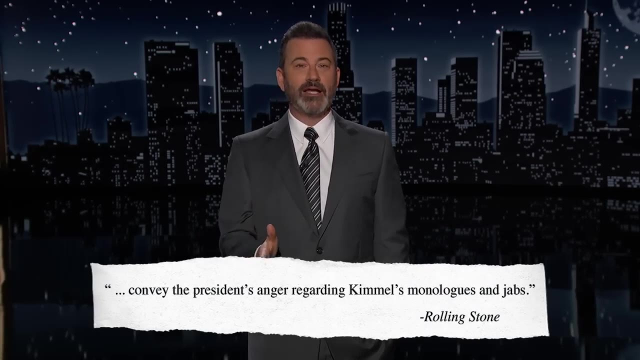 to tell them to rein me in. The report says at least two calls were made from the Trump White House, to quote: convey the president's anger regarding Kimmel's monologues and jabs. In other words, President Karen demanded to speak to my manager. 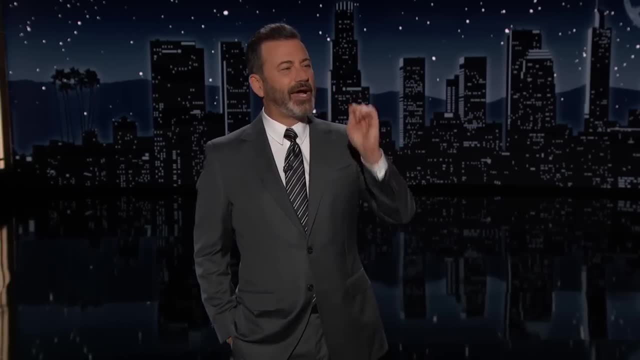 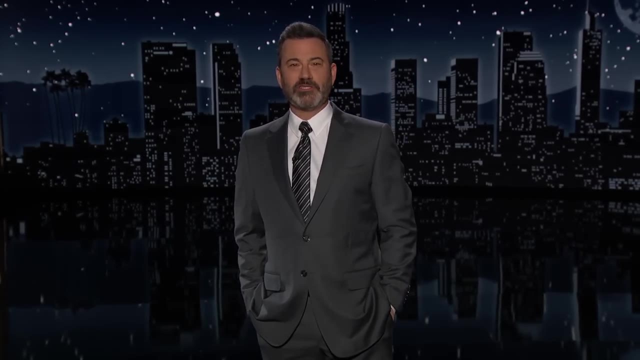 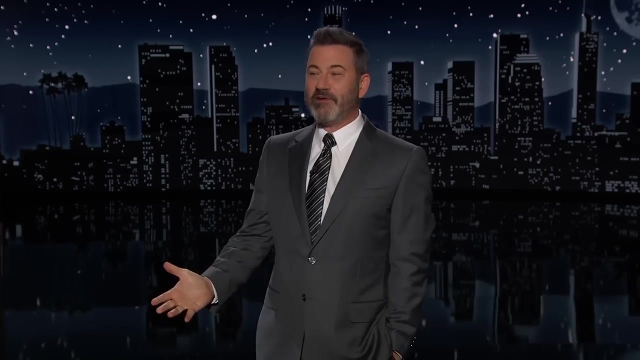 And you'd think the guy who fathered Eric and Don Jr would know how to handle jokes, but I guess not. The article says news of these calls spread around the corridors of power in Washington. Wow, what a plot twist. The first time Donald Trump ever tries to stop someone from talking about him on television- and it's me. 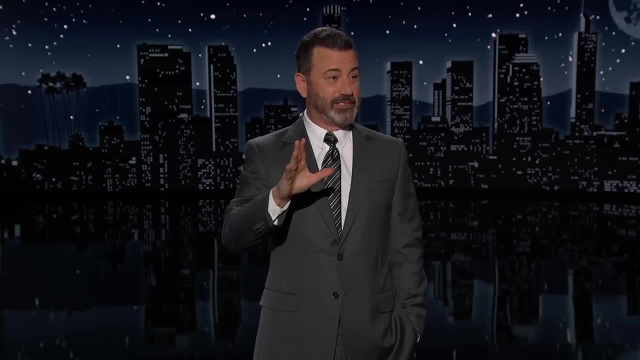 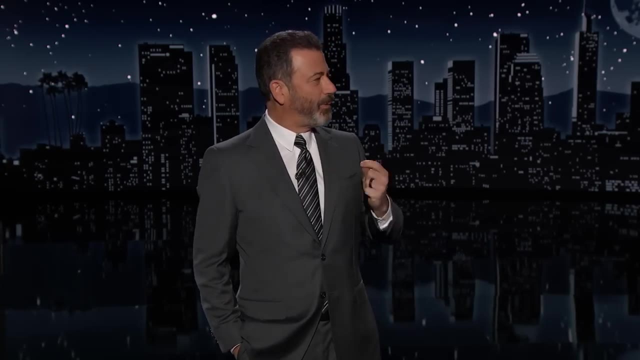 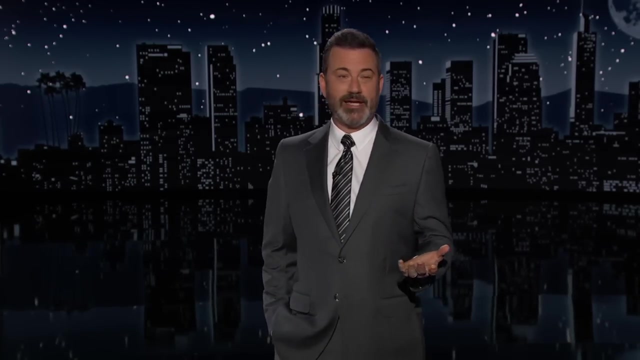 Usually, when he wants somebody to stop talking about him, he pays them $130,000, but he wanted me to do it for nothing. I wonder what it was specifically that sparked his trumper tantrum. I wonder what it was he found so objectionable. I don't know. maybe it was the time I had Stormy Daniels look at a plate of carrots to size them up, and she picked the little one. 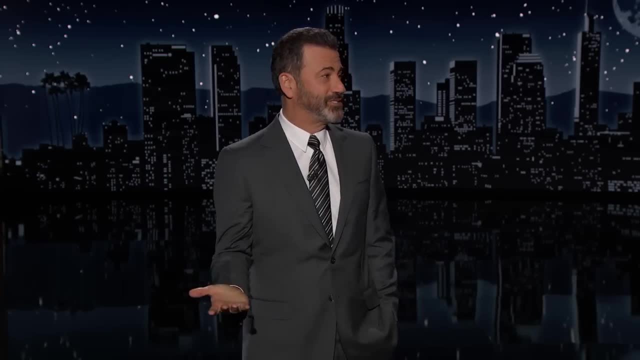 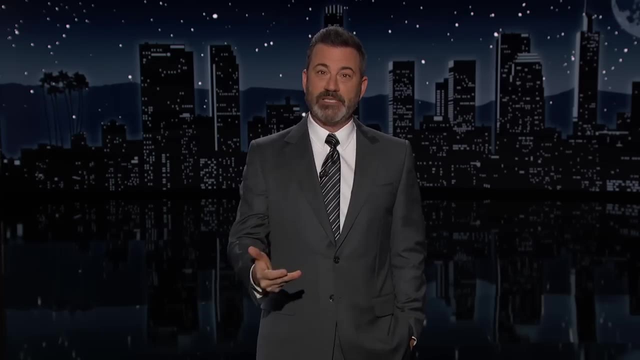 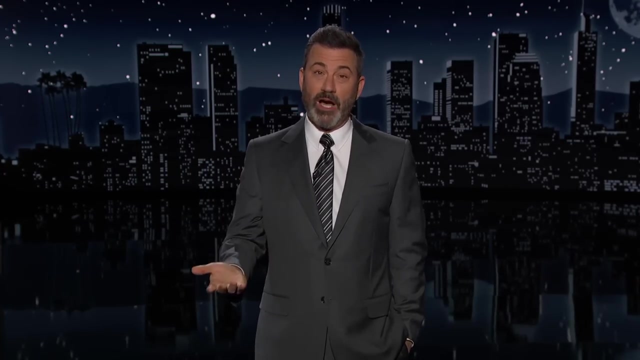 I don't know, maybe it was one of the nicknames I went. it was going through like Tanny Soprano, Nostra Dumbass, Emperor Palpatine, Hands Mara, Lardo, King, Tootin' Con Man, The Hydroxy Horror Picture Show, Pumpkin McCornhumper, Grabass, Grandpa Orange, Julius Caesar, Coludacris, Flabios, Freddy Krueger, The Tandalorian, Liger Woods, Cuedon, Dictator Tot. 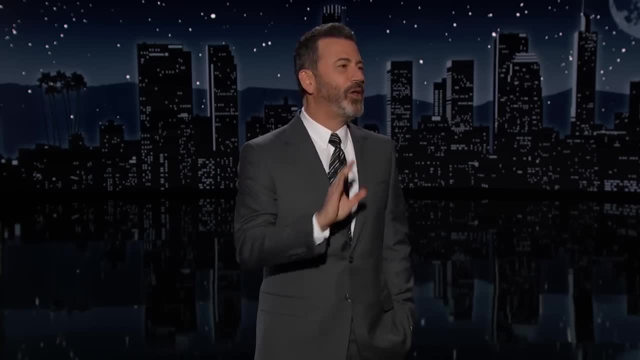 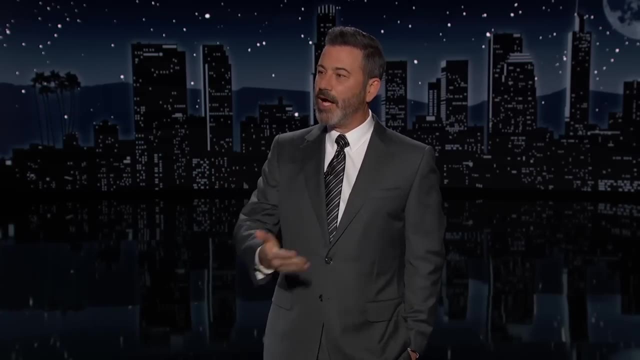 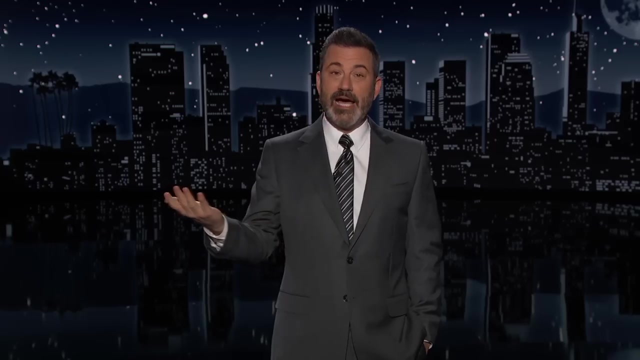 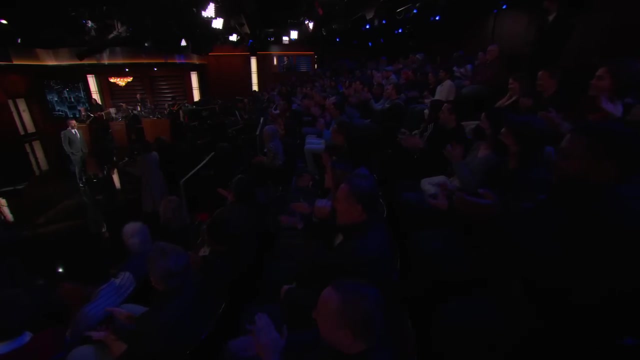 Just give me. I only have, I only have a hundred more. okay, Quick Broke Home Over Uncle Scam, Fibaracci The One Terminator, Chocolate Mussolini, YMCA Hole, The Recount of Monte Cristo, Daddy Bone Spurs or George Washington- maybe that was the one- because, wow, what a fragile little snowflake, what a blowhard. 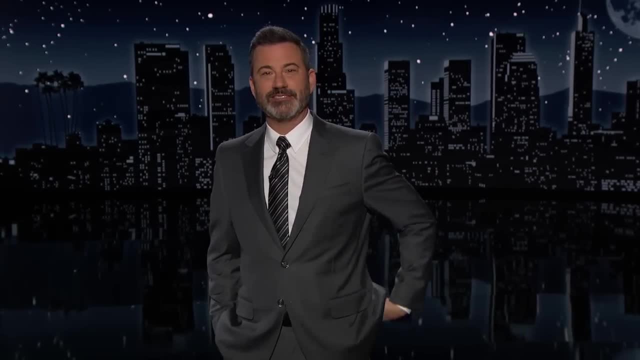 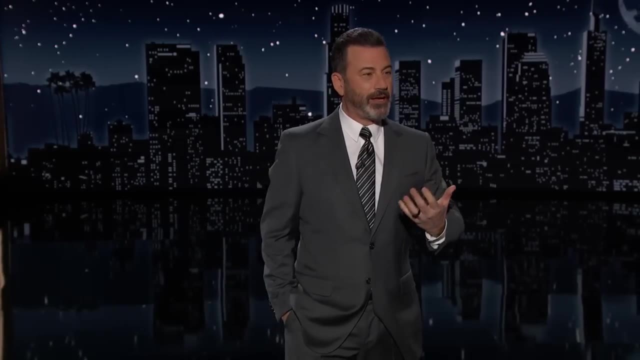 He's a blowhard. He's a blowhard and a snowflake. He's a blowflake is what he is. He should change the hats to say Make America Wine Again- Mawa, because when you think of all the people I regularly make fun of, it's a lot of people. 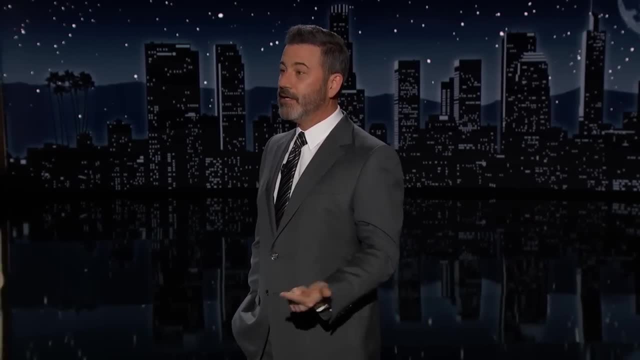 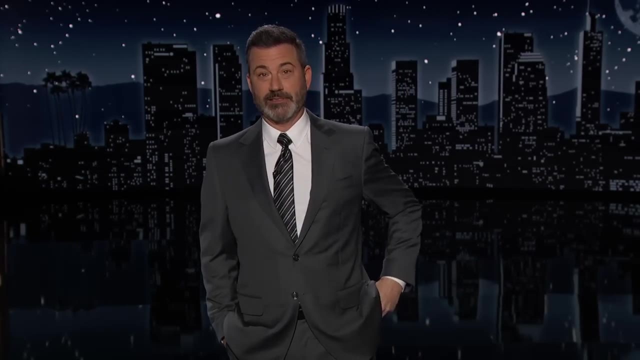 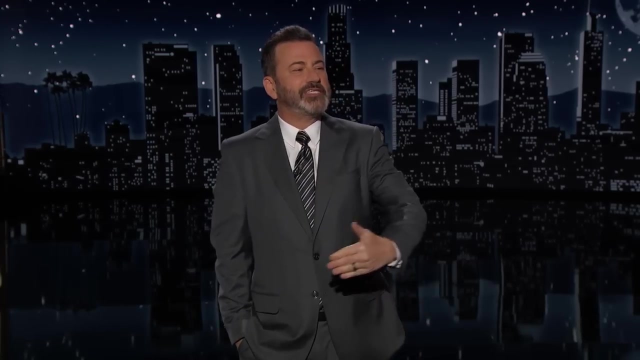 The only two who've tried to stop me are Donald Trump and Marjorie Taylor Greene, who actually called the cops on me. I'm in front of OJ a thousand times. he hasn't tried to kill me once. And this guy, Donald Trump, all he does is make fun of. he makes fun of disabled journalists. 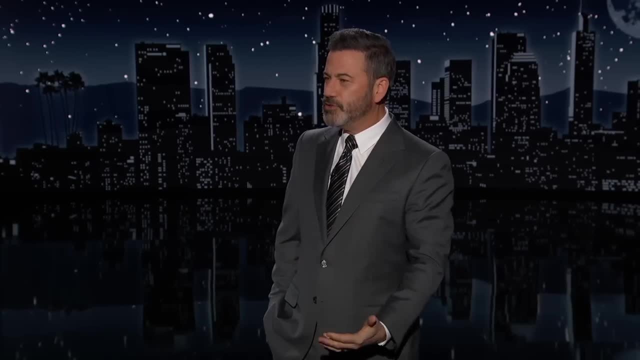 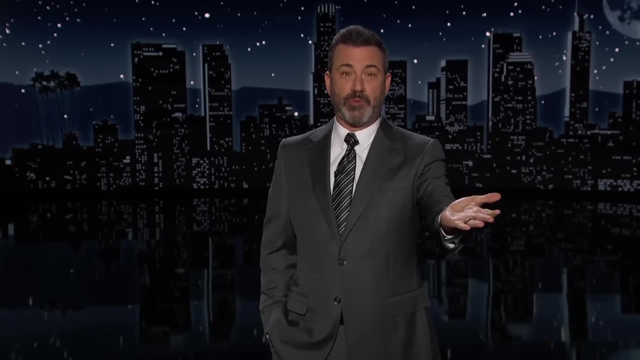 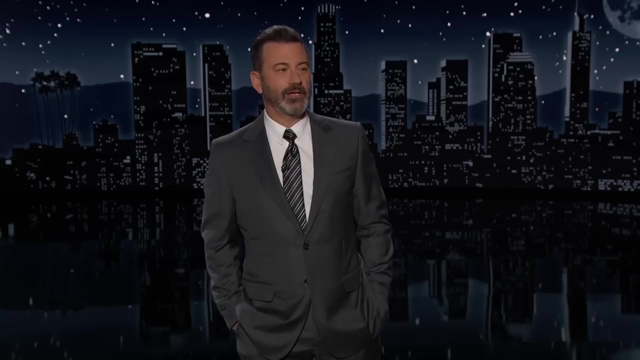 he calls our veterans, prisoners of war, even losers. he insults his opponents, his friends, his family. But if I point out that he's so fat they renamed the plane Air Force Wonder Bread, I'm the bad guy, I don't know it's. maybe you know what. maybe this is why Donald and Melania sleep in separate bedrooms. 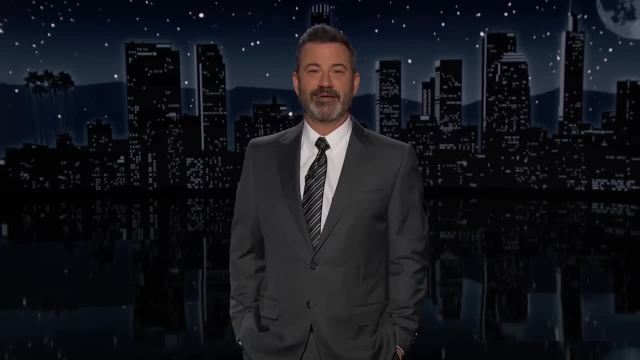 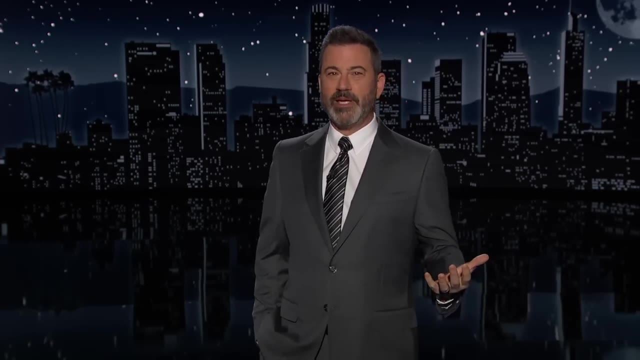 She was laughing too hard at my monologue at night. But really, joking aside, this is a blatant abuse of power. I wonder Fox News- you know they're always screaming about censoring comedians- Will they defend me on this? 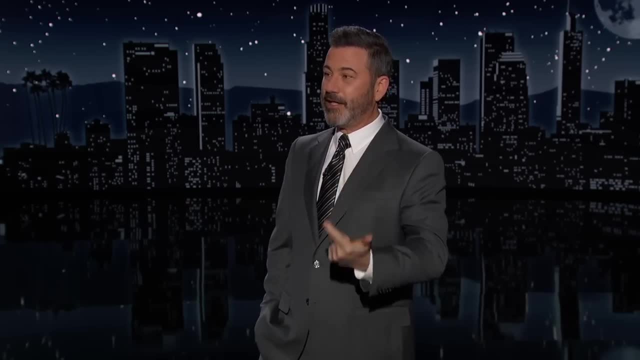 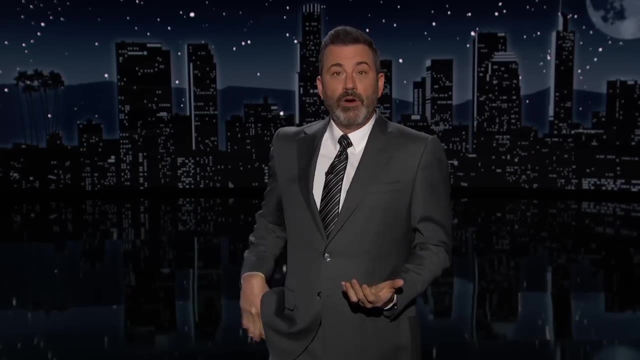 I doubt it. We have a First Amendment right that Americans are a hell of a lot braver than Donald Trump died for, and it's especially hypocritical coming from someone who claims to be the bigliest anti-censorship defender of free speech. 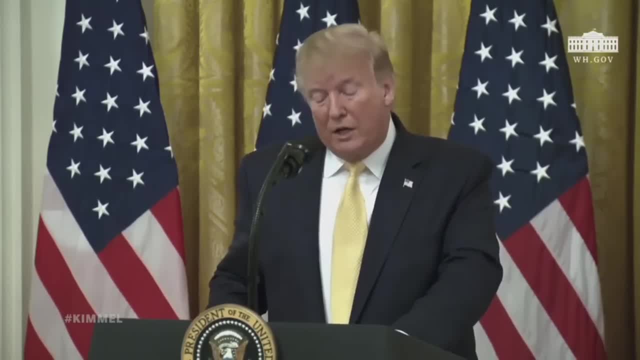 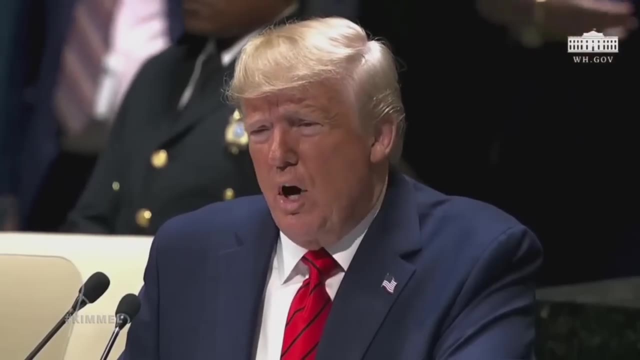 Today I'm directing my administration to explore all regulatory and legislative solutions to protect free speech and the free speech. We have free speech rights of all Americans And we're here today to discuss protecting Americans from censorship. We will uphold the right of free speech. 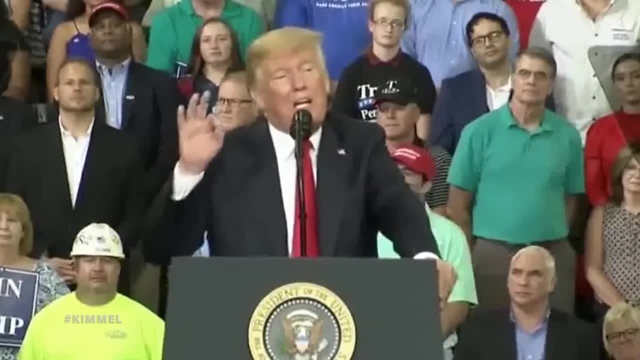 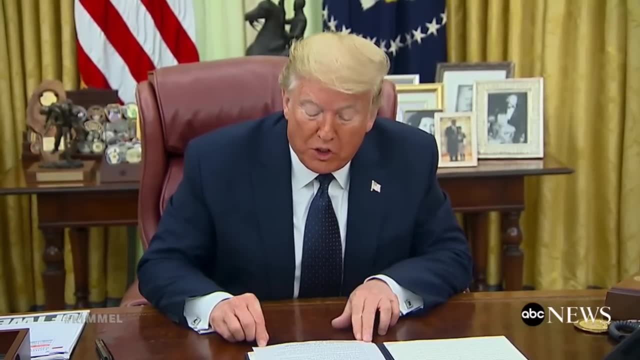 We as a country cannot tolerate political censorship. We will always, always protect free speech. The censorship and bias is a threat to freedom itself. Free speech is a bedrock of American life. We believe in free speech Censorship. 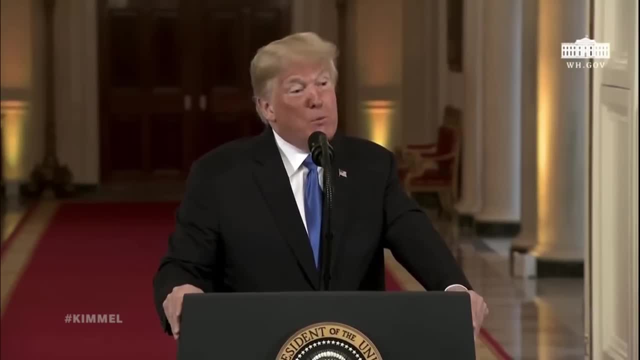 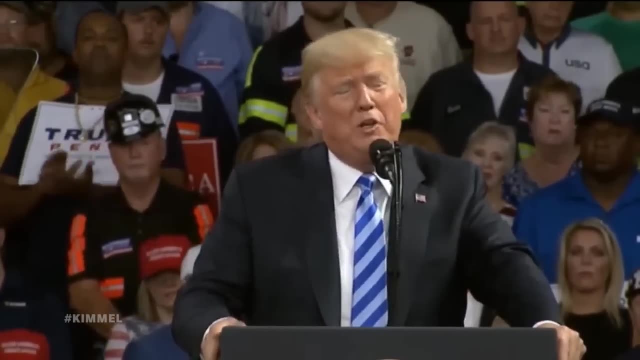 Free speech, Censorship, Free speech, Censorship- Believe it or not, someone that really likes free speech. You can't have censorship. You can't pick one person and say, well, we don't like what he's been saying. 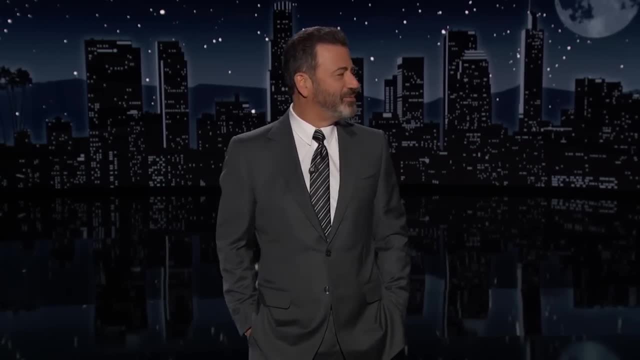 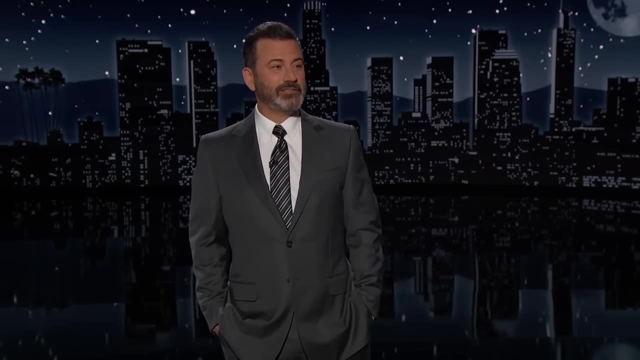 He's out. It's very interesting. It's almost like he's a hypocrite, you know, And you know what else is a shame. Jim Jordan just had his big congressional hearing on the weaponization of the federal government and I couldn't be there to testify. 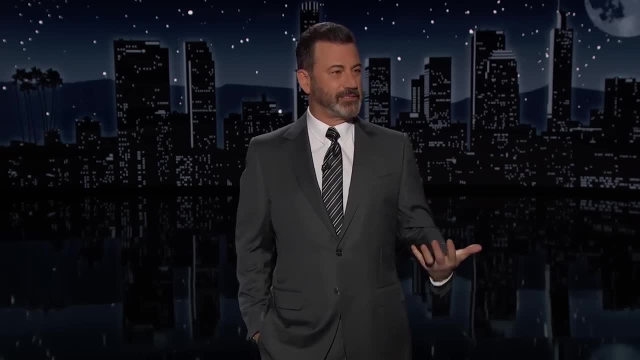 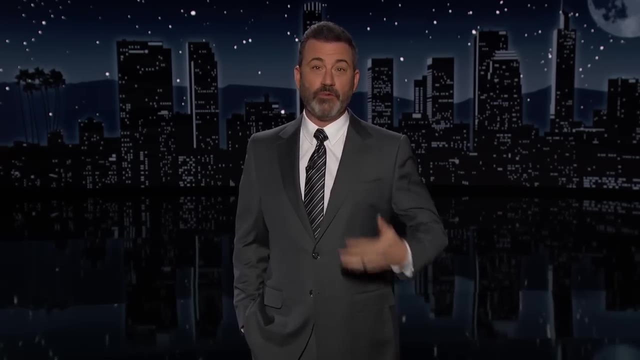 about a president of the United States who abused his authority to silence someone who disagrees with him and tried to muzzle free speech. I'm so sorry, Jim. I would have been happy to help with that And as for Trump, you know if you 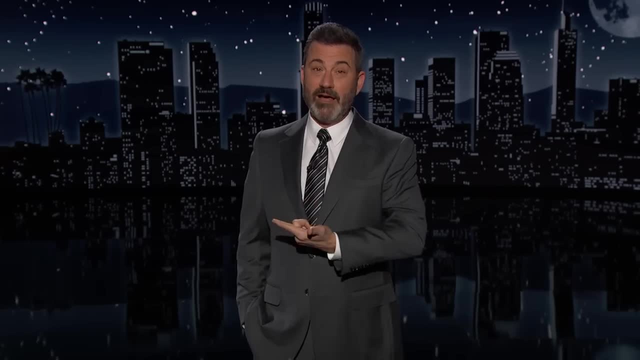 want to come on the show to tell me to be quiet yourself. we still have that arcade claw machine that my pillow guy got in. You can climb inside and say whatever's on your delicate little mind, OK? We're now less than two weeks away from the Oscars. 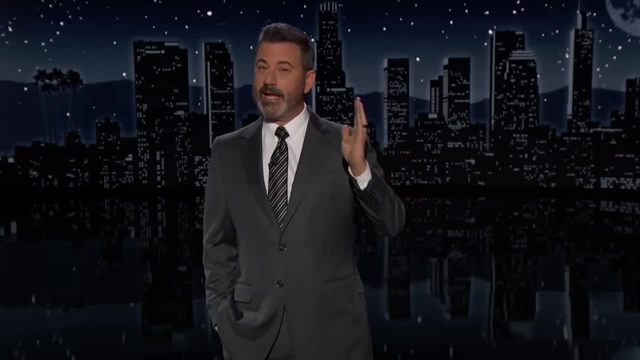 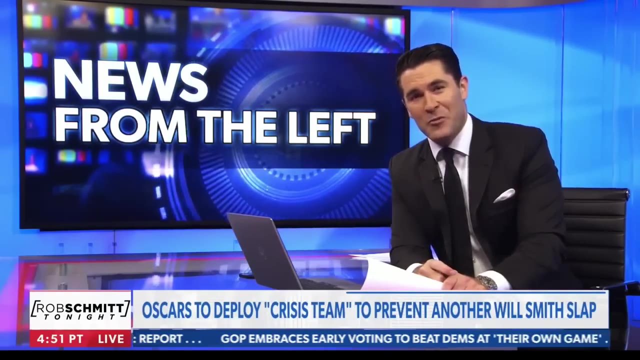 The Oscars are on Sunday, March 12,, here on ABC, And I tell you you can really feel the excitement starting to build. This year's Oscars will now feature a crisis team, in case Will Smith shows up again. Academy Awards are scheduled for March 12.. 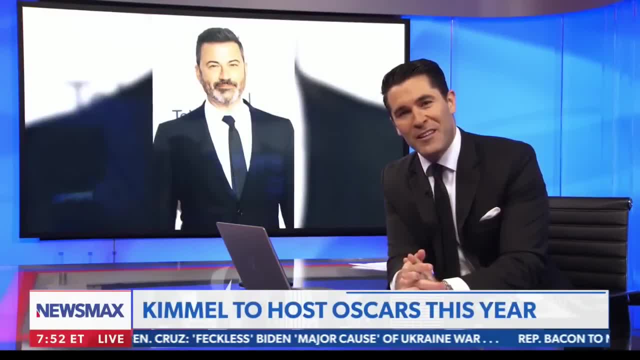 Jimmy Kimmel will host this year. That means it's going to suck. You don't have to watch it. Just watch me on Monday and we'll make fun of it together. Well, he said it's going to suck. I think you missed that. 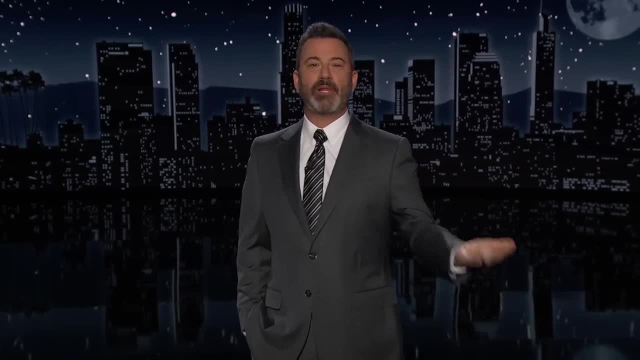 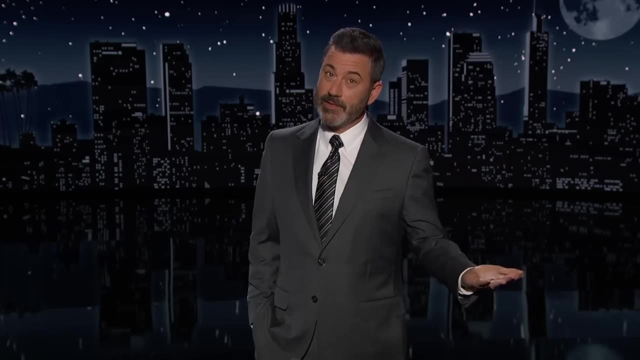 I don't know, that's not very open-minded. OK, maybe you don't like me, but what about Cate Blanchett's hauntingly beautiful portrayal of a lesbian orchestra conductor in the three-hour German and English drama Tar? You're only cheating yourself, OK. 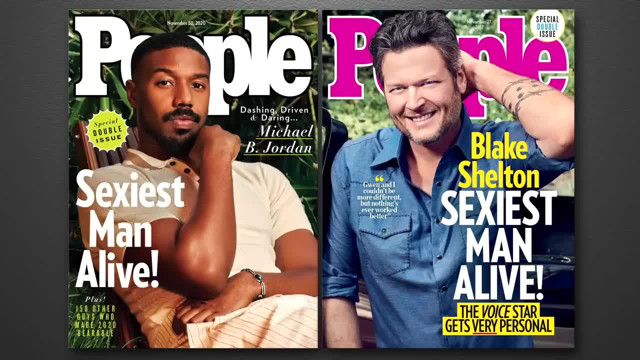 Tonight on this show, we have not one, but two of People Magazine's Sexiest Men Alive: Michael Jordan, who was the sexiest in 2020.. And Blake Shelton, who was Sexiest Man Alive in 2017.. And technically, there were three Sexiest Men Alive. 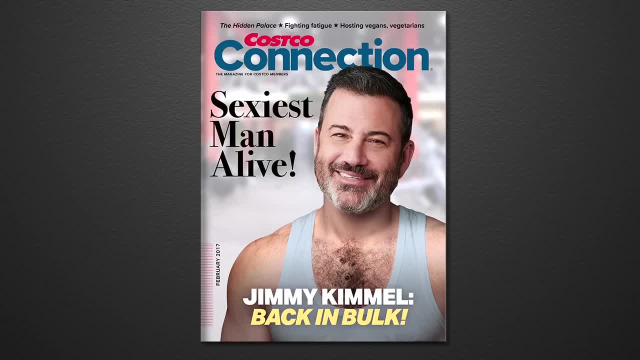 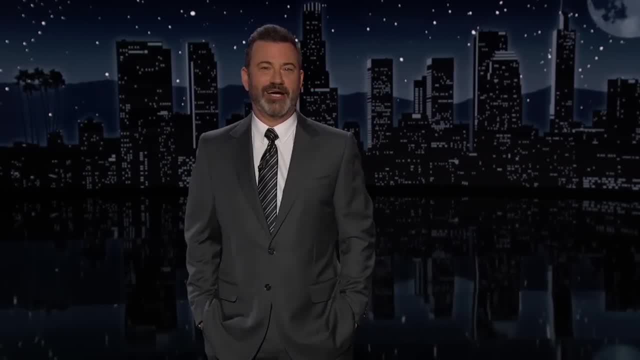 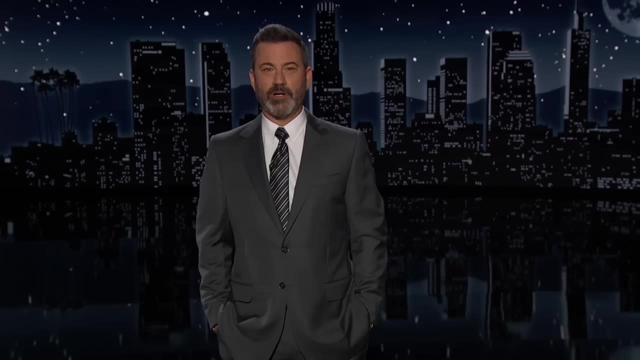 if you count my cover of Costco Connection magazine, which is So, I think that's a record. Either way, stay tuned for Sexy tonight. Kanye West has been out of the spotlight For a couple of months now. Adidas parted ways with Kanye in October. 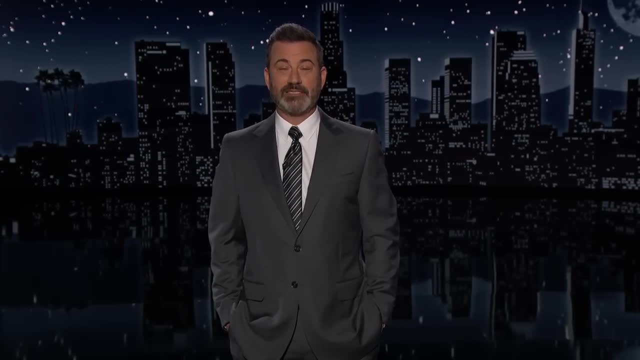 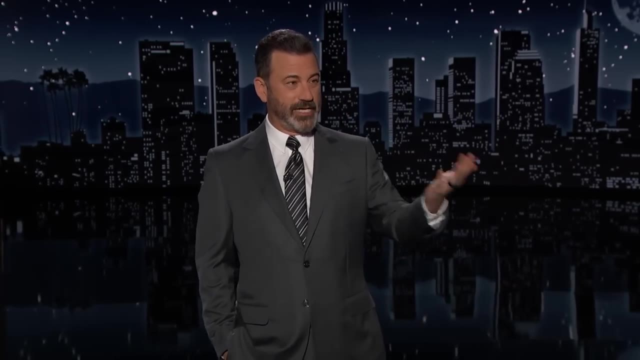 And now they're stuck with $500 million worth of back stock Yeezys. These are Yeezys that they were planning to sell, but they promised not to profit off Ye and his shoes after his anti-Semitic tirade. So Adidas now has to figure out what. 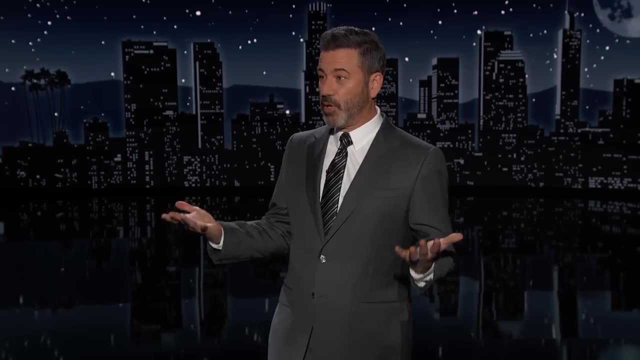 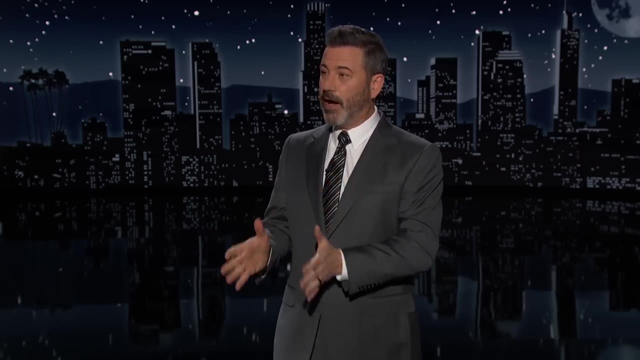 to do with all of these shoes. One of the options is to burn them, which I don't know. seems like burning a pile of shoes is historically a bad look for Germany in general. The other option would be to donate them to disaster relief organizations. 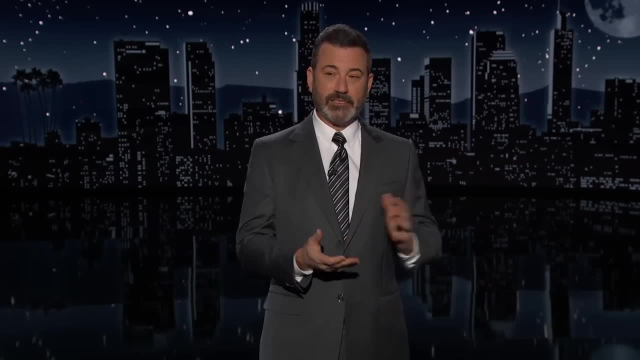 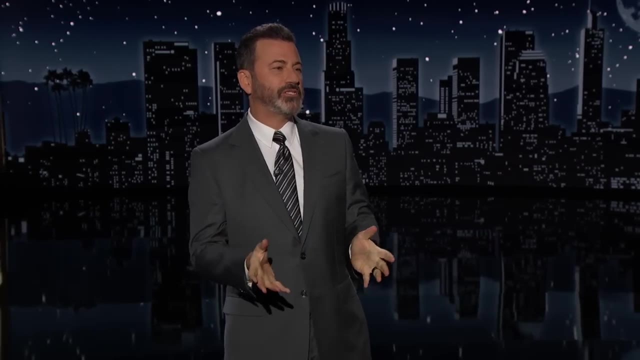 to help people in places like Turkey and Syria. I don't know, It's a tough call. What would Yeezys do in this situation? The other problem with the shoes is that they look like well this, So they look like what happens if you put a pair of Crocs. 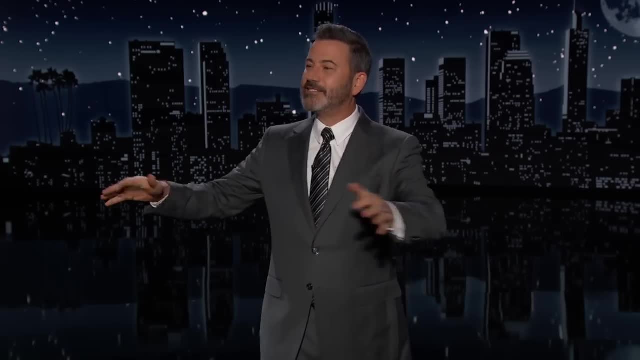 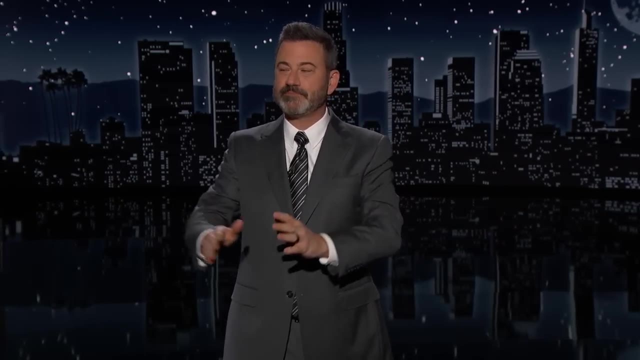 in the microwave. Maybe what they do is they tie all the shoes together, make a giant raft and then push Kanye out to sea on it. You can believe it. You can probably use a raft right now, Far West Valley where he lives. they. had more than 10 inches of rain over the weekend. My house- we just keep getting the leaks repaired. It rains, it leaks. We get it fixed. They say, OK, it's all good now. Then four months later it rains again. 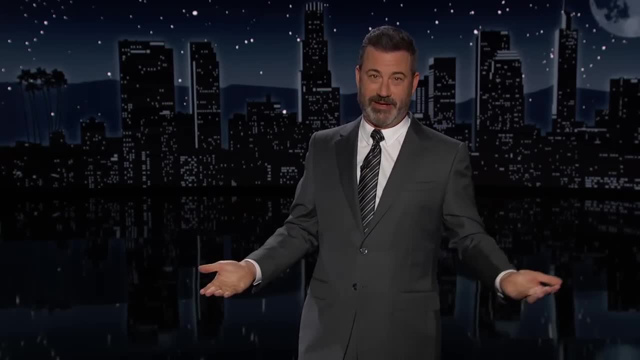 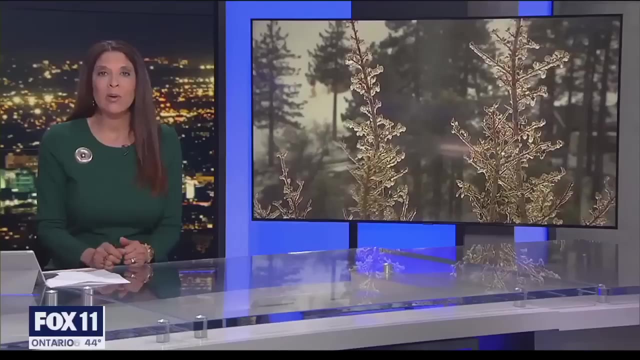 and we got buckets all over the floor and all the same It even snowed here this weekend, which is all actually very exciting for our local weather people who really never get to report anything ever. Mr Fajardo is in Wrightwood with us. 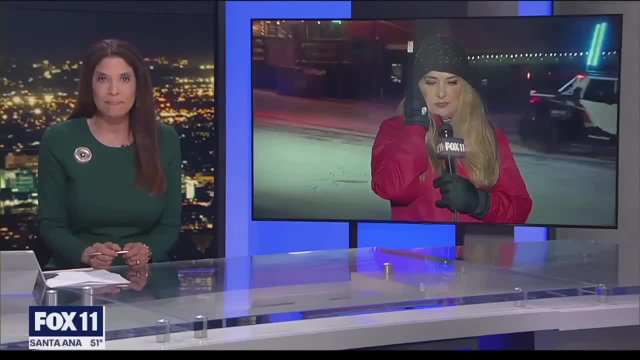 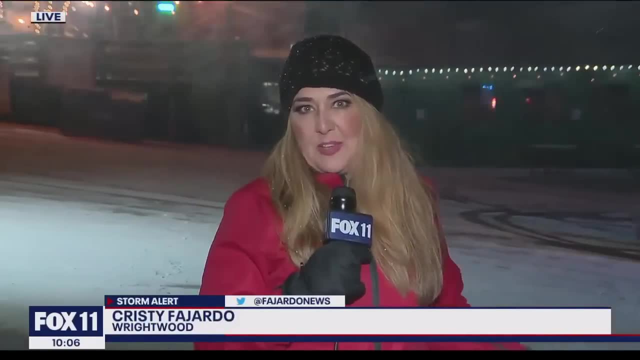 He's in Wrightwood with our continuing storm coverage. Kristi, Yeah, you know I'm sorry I can't hear. you Probably can see what's going on behind me. There's somebody doing donuts in the snow trying to get our attention, apparently. 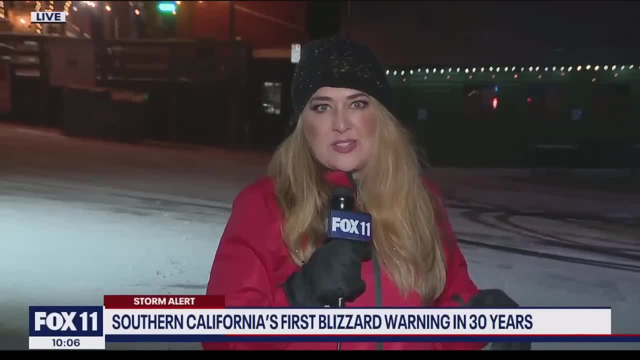 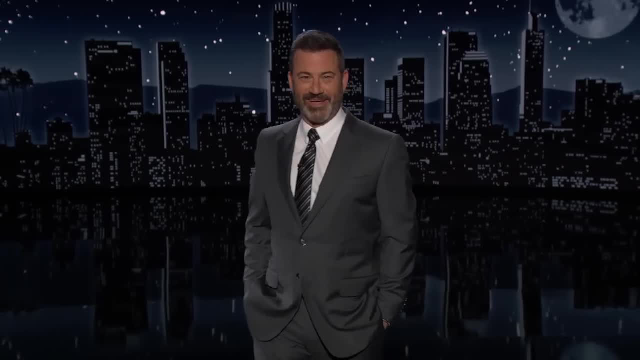 But I can tell you we're starting to see some snow flurries And enough of it has fallen that it's starting to accumulate here on the ground. Yeah, that's what we want: to look at the ground. We don't want to, not the monster. 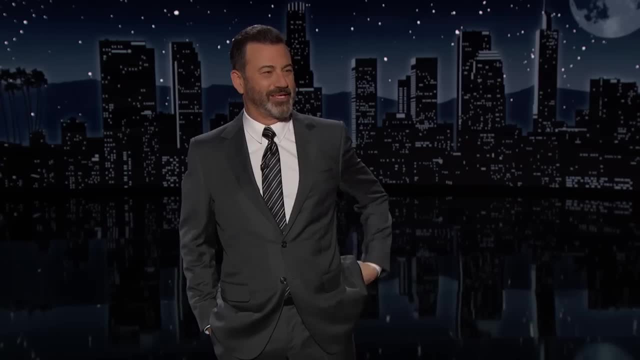 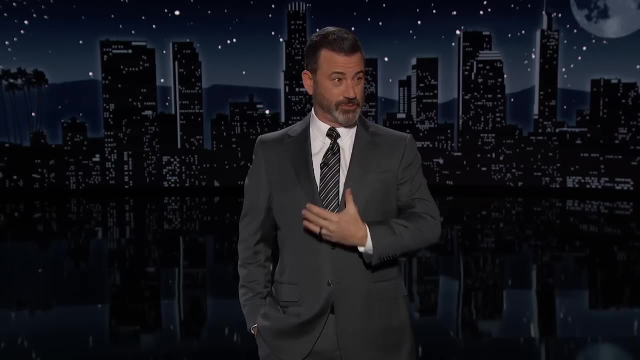 but the monster truck from Star Wars doing snow donuts. We want to look at the ground. We are not prepared for rain here. We just don't know what to do when it happens. So what we do do is we just drive around like there's nothing unusual happening at all. 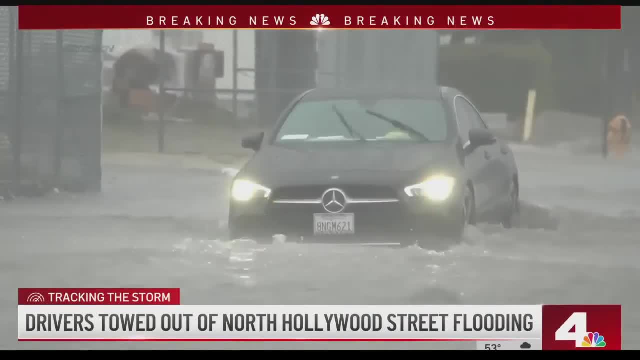 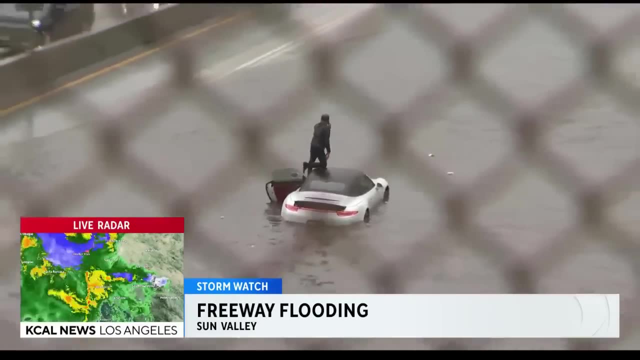 This is right next to Hollywood Burbank Airport. Nearly a dozen cars were stuck in the water as they tried to make it across the road. This driver, this Porsche, became stranded on the roof of his convertible after he got stuck in the floodwaters on the 5 freeway. 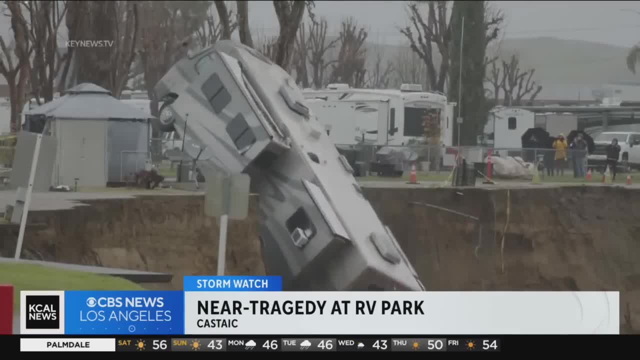 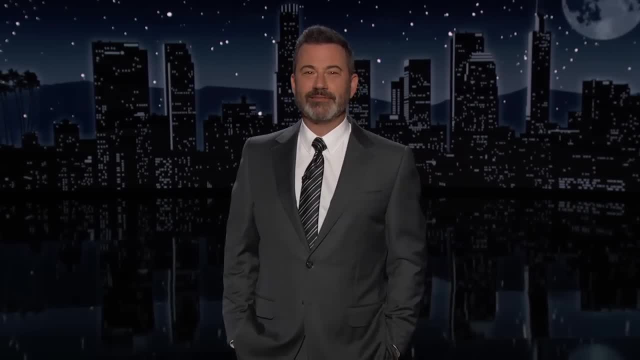 Take a look as this RV just slides into the river. At the Valencia Travel Village RV Resort, two other RVs went straight to the Santa Clara River. Isn't it great that we have video of everything now, In the old days, when you would lose your RV. 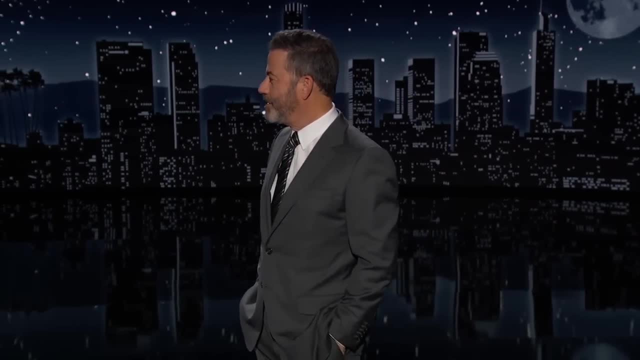 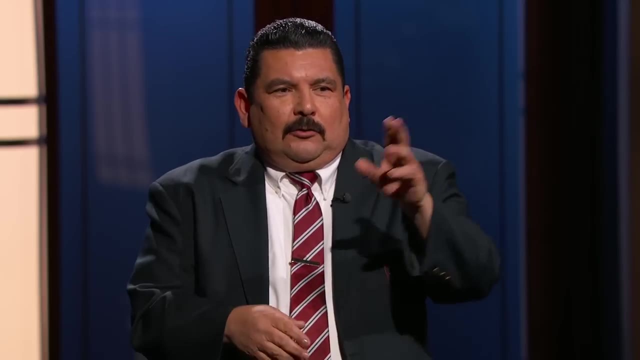 you'd have nothing to show for it. Is everything OK at your house, Guillermo? Yeah, we lost the power for like two or three hours. Oh, you had no power. Yes, You have a generator. No, we went across the street with the neighbors. 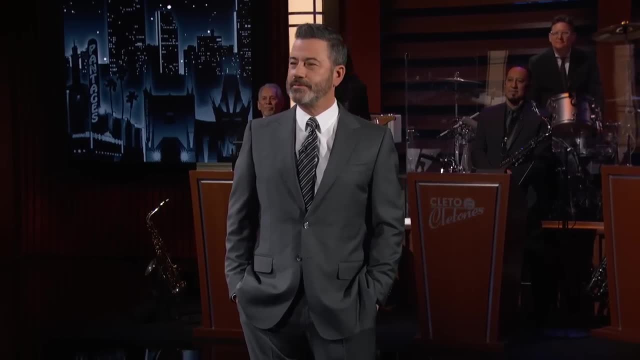 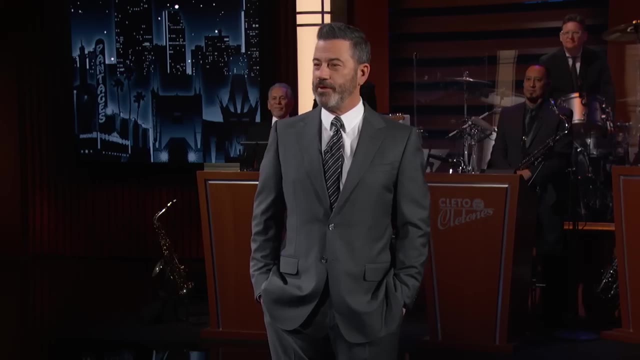 They do have one. Oh, the neighbors had a generator, Yeah, and they let us stay for a couple of hours. Now are you going to get a generator? Yeah, I'm planning to. yes, You are OK, But the neighbors will come over to your house. 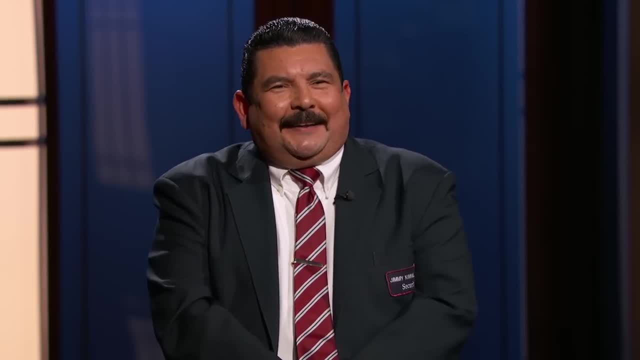 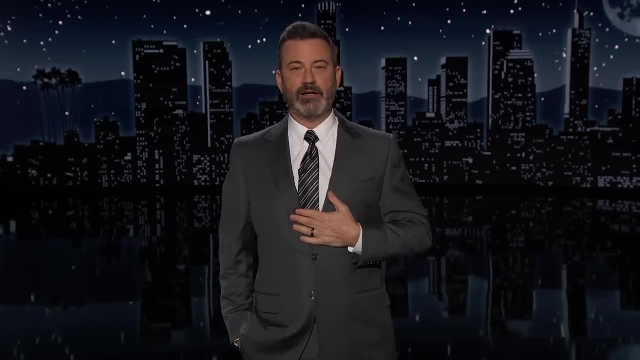 Yeah, so, yeah, it's OK, It's OK, all right. You know, nothing's easy anymore. Even the mundane moments of daily life can be very stressful, And so that's why I am so grateful to get help, not from a friend or a neighbor or a therapist. 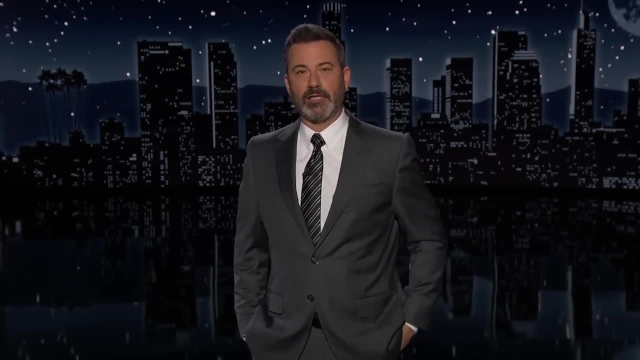 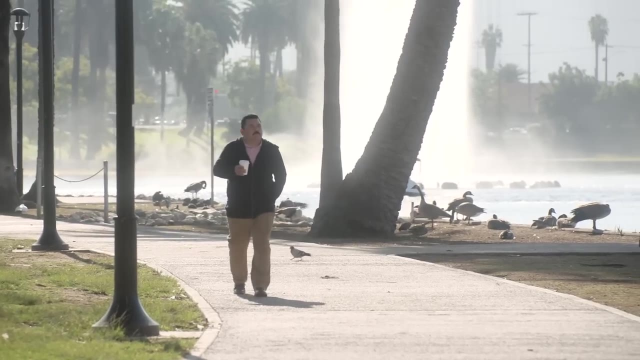 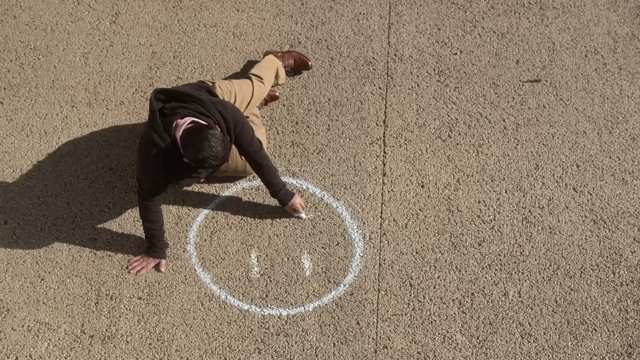 but rather from where God intended us to get it: from a bottle. Sometimes a good day feels like a bad day. Sometimes the things you enjoy just aren't fun anymore. Sometimes sadness seems like the only choice, But it doesn't have to be. 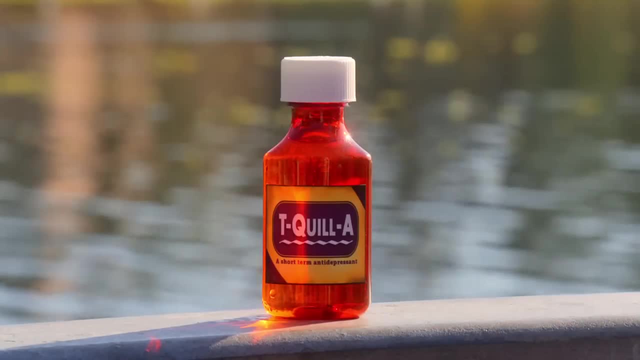 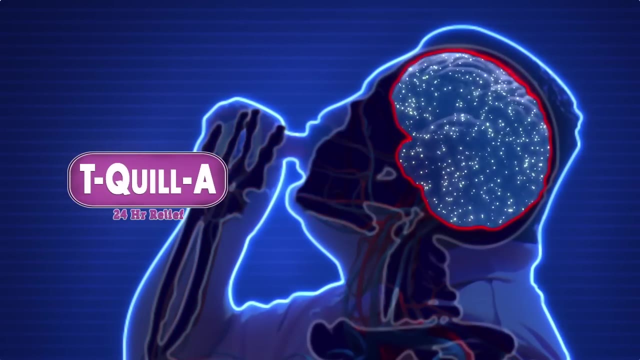 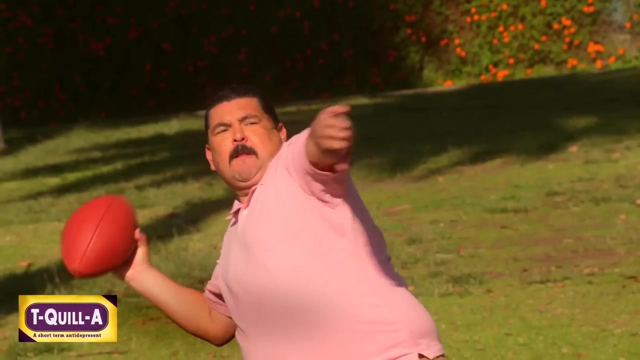 Get help. Get T-Quilla. T-Quilla is taken orally as needed and works almost instantaneously, triggering dopamine production in the brain, so you can feel better and get back to living life again. The side effects of T-Quilla mean. 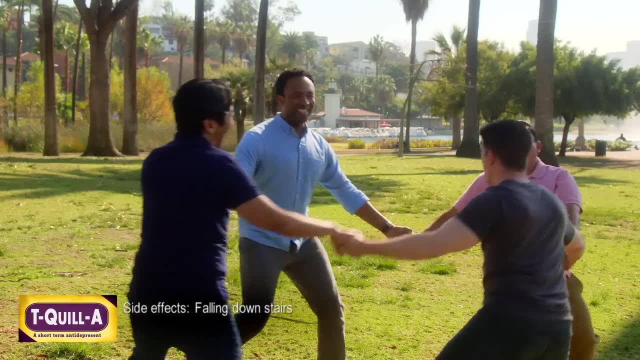 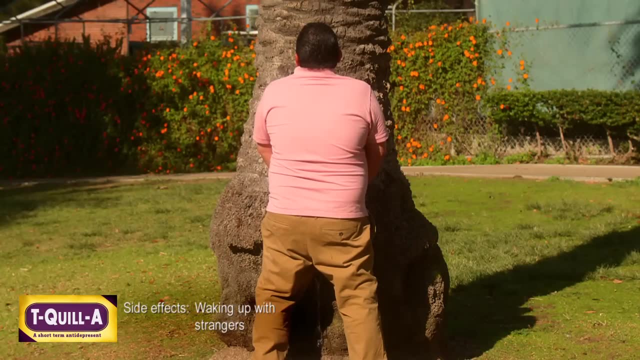 that it may include headache, nausea, dehydration, falling downstairs, falling off tables, falling off of chairs, running naked in the plexiglass trying to fight garbage cans, breaking up with strangers and leaving your ex passionate voicemails at 4 AM.